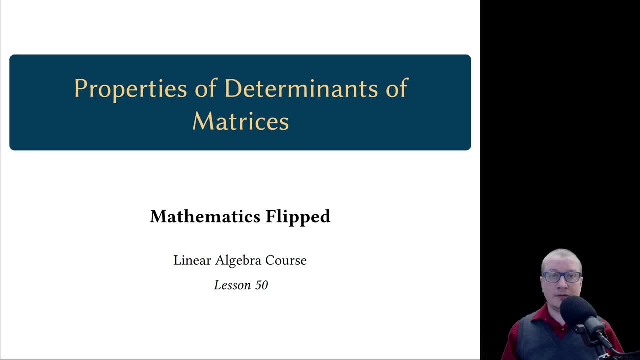 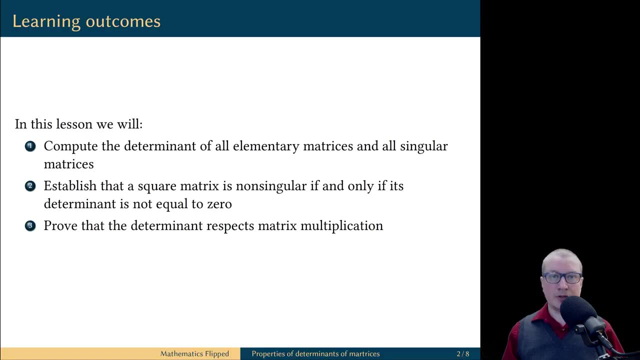 Welcome friends. Igor is here and in this video we will understand why it is useful to know the determinant of a matrix. In this lesson we will compute the determinants of all elementary matrices and all singular matrices. We will establish that a square matrix is non-singular if, and only if, 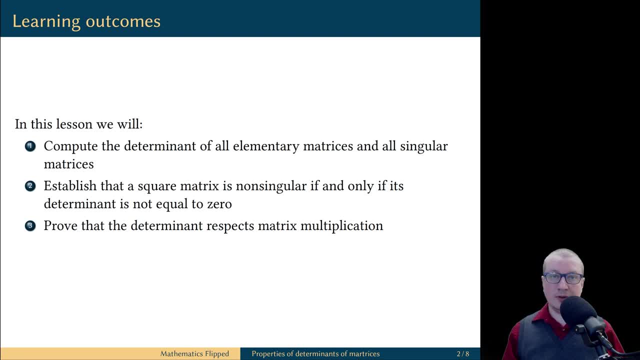 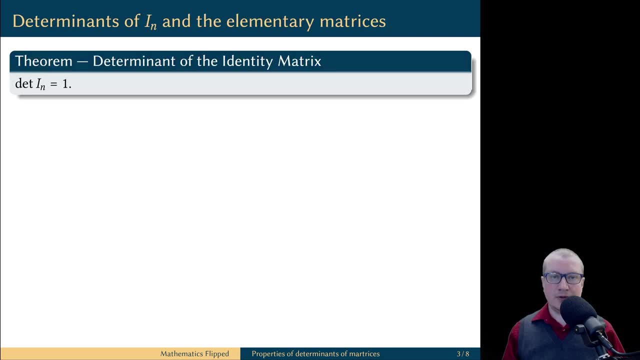 its determinant is not equal to zero, And we will prove that the determinant respects matrix multiplication. Let's get started. First simple observation is that the determinant of the identity matrix is equal to one. That is because the identity matrix is in upper triangular form. 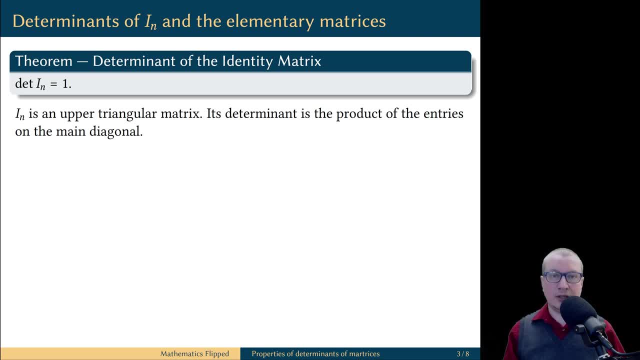 and we already discussed that the determinant of a matrix in upper triangular form is equal to the product of its entries on the main diagonal. This allows us to compute the determinants of all elementary matrices. If an elementary matrix is not equal to zero, then the determinant of a matrix 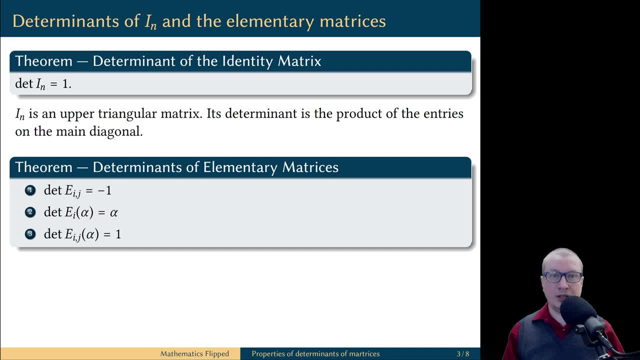 was obtained by swapping two rows of the identity matrix, Its determinant is negative one. If an elementary matrix was obtained by multiplying one row of the identity matrix by scalar alpha, then its determinant is equal to alpha, And if an elementary matrix was obtained by multiplying 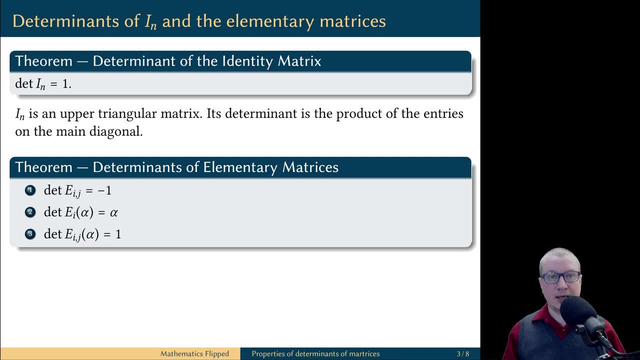 one row of the identity matrix by scalar alpha and adding the result to another row, then the determinant of this matrix is equal to one. This result is a trivial consequence of our earlier observations on how performing elementary row operations affects the determinant. For example, if we swapped the two rows of the identity, 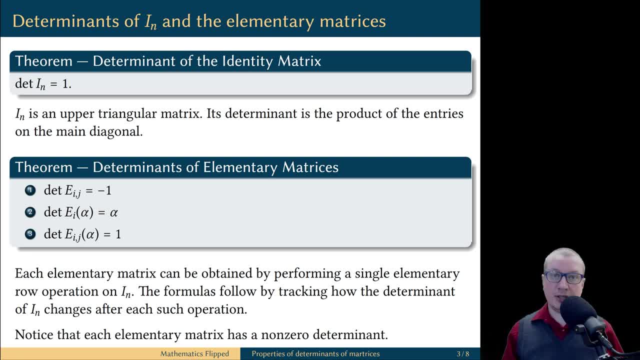 matrix to get the elementary matrix, then we have changed the sign of the determinant of the identity matrix, but the determinant of the identity matrix is one. therefore the determinant of the corresponding element of the matrix is negative one. But the most important piece of information, 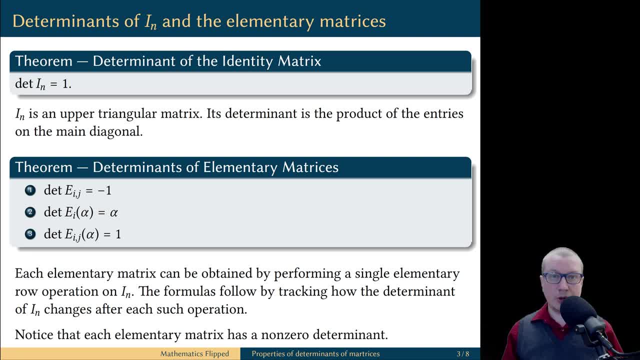 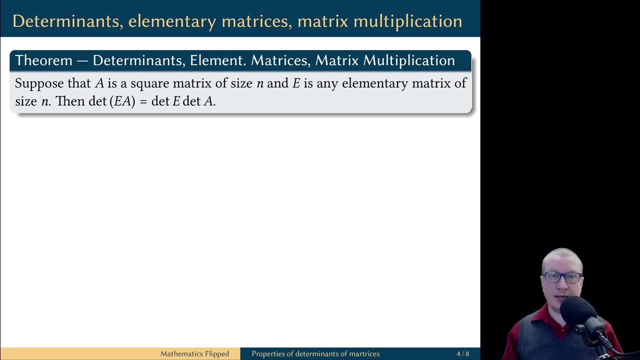 for us from this result is that the determinant of each elementary matrix is not equal to zero. Remember, in the second type of an elementary matrix, alpha has to be a non-zero scalar. And now let's prove that. if you take a square matrix A and multiply on the left by an elementary 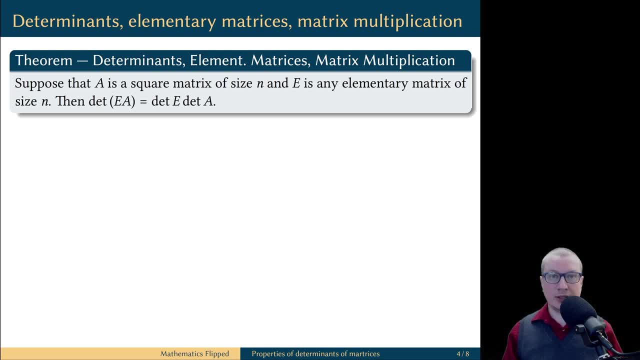 matrix E, then the determinant of the matrix product is equal to the product of the individual determinants. We will show why it holds for each type of an elementary matrix. First, suppose that we deal with an elementary matrix which was obtained by swapping rows i and j of the identity. 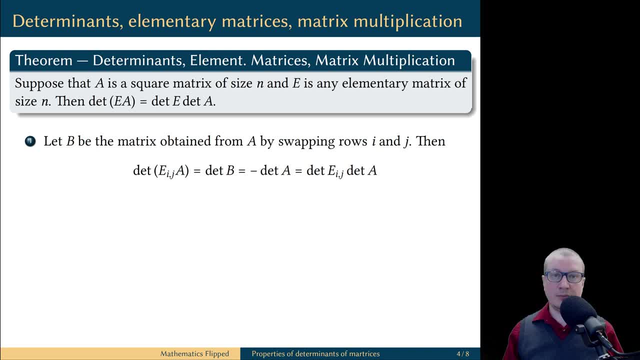 matrix. Let's also construct a matrix B by performing this same row operation on the matrix A. In the previous video we discovered that this matrix B can also be obtained by multiplying matrix A on the left By this elementary matrix. So the determinant of the elementary matrix times matrix A is equal. 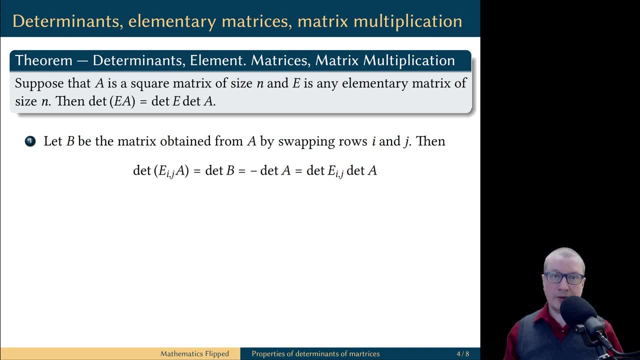 to the determinant of the matrix B. On the other hand, the matrix B was obtained by swapping two rows of a matrix A. Therefore, determinant of matrix B is negative determinant of the matrix A. The last step is to recall that the determinant of the elementary matrix, obtained by swapping two. 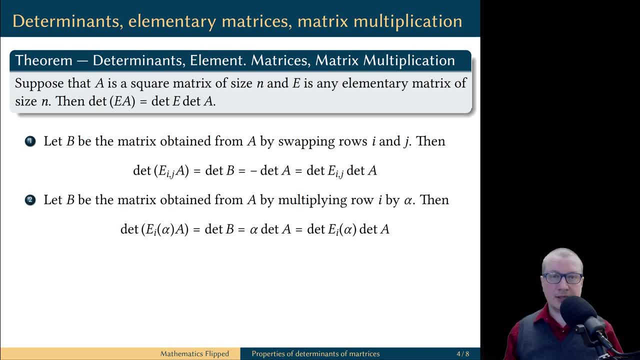 rows is negative. one Second. let's look at an elementary matrix which was obtained by multiplying row i of the identity matrix by scalar alpha. Let's perform this same row operation on the matrix A and the result is the matrix B. Same idea as in the first part. The matrix B can be expressed as a product. 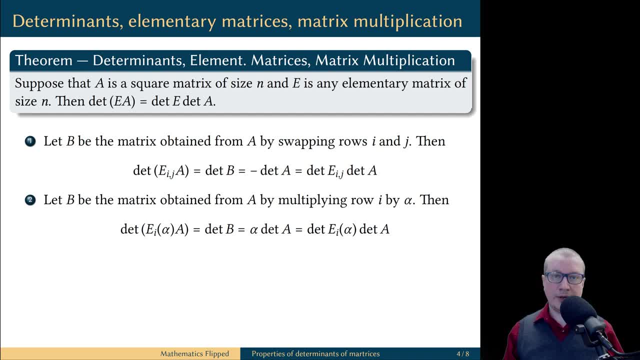 of the elementary matrix and the matrix A. On the other hand, matrix B was obtained from A by scaling one row by alpha. therefore, the determinant of B is equal to the determinant of A multiplied by alpha. The last piece of the puzzle is to recall that the determinant of an elementary matrix 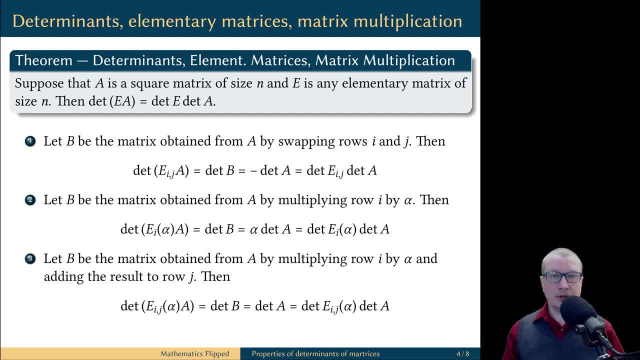 of this second type is exactly alpha. Third, let's say we have an elementary matrix which was obtained by multiplying row i of the identity matrix by alpha and adding the result to row j. Let's also apply this same row operation to matrix A to produce matrix B. 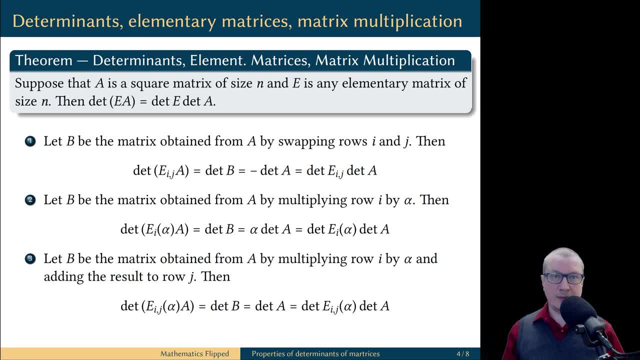 Then this matrix B is the product of the elementary matrix and matrix A. On the other hand, because the matrix B was obtained by applying the row replacement operation on matrix A, they have the same determinant. The last observation is to recall that the determinant of an elementary matrix of type 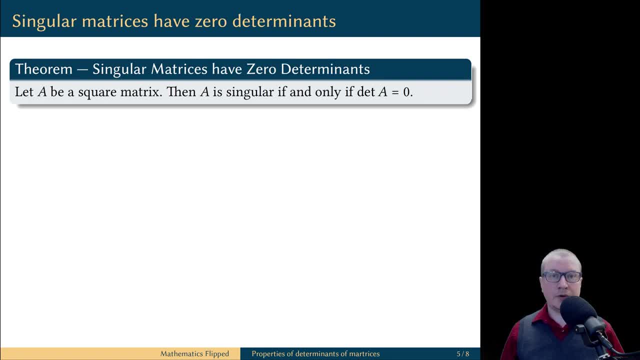 3 is equal to 1.. And now we are ready to play. Let's try to prove that a square matrix is singular if, and only if, its determinant is equal to zero. This is an if and only if statement, and therefore we need to prove two implications. 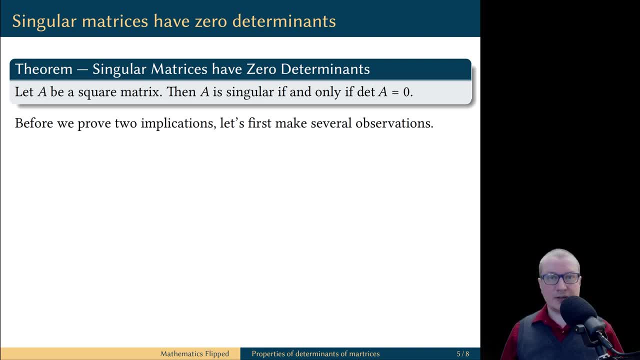 But before we get to that part, let's make some observations. We have a square matrix A and let B be the reduced row echelon form of this matrix A. This means there is a sequence of elementary row operations. Let's make some observations. 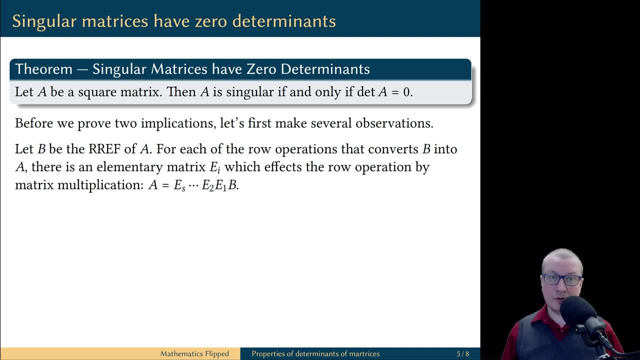 In this sequence we can see that B transforms A into B, but then, by reversing this sequence of row operations, we can also transform matrix B into the matrix A. So for this sequence of row operations which transforms the reduced row echelon form B into 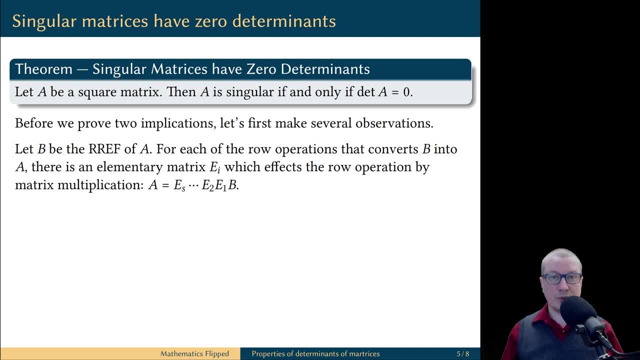 the matrix A, we will record the sequence of corresponding elementary matrices And then performing this sequence of row operations on the matrix B is equivalent to B to multiplying this matrix on the left by the corresponding sequence of elementary matrices. The result of this is the matrix A. Now let's compute the determinant of A. It is equal. 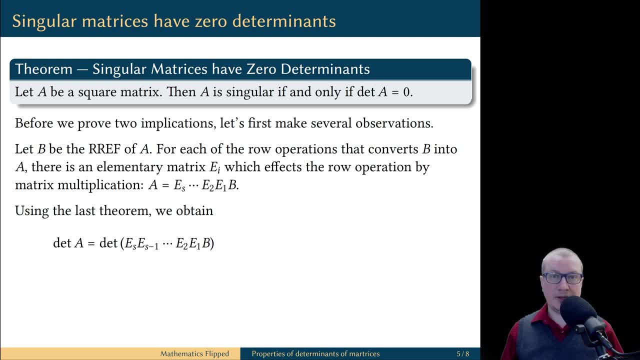 to the determinant of this long product of matrices. and let's think of this long product as follows: It is the leftmost matrix ES multiplied by the rest of the product. By the last theorem we just proved, this is equal to the determinant of the matrix ES multiplied by the 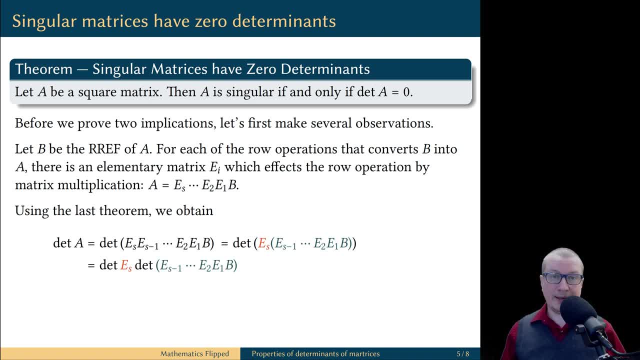 determinant of the other matrix. But then we keep doing this. We chip away one leftmost elementary matrix at a time, We keep applying this same theorem and this is what we'll get. So the determinant of A is equal to the product of all these determinants. But let's recall: 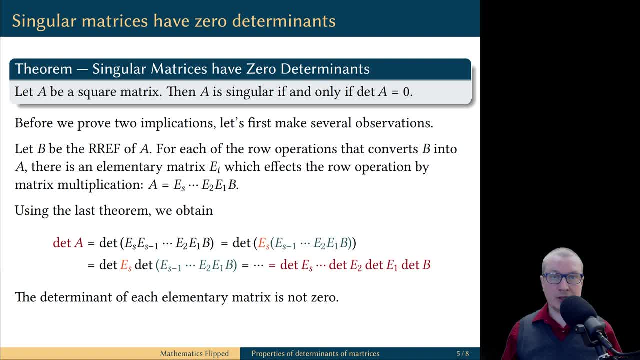 that the determinant of each elementary matrix is not equal to zero. This means that the determinant of the matrix A is equal to zero if, and only if, the determinant of the matrix B is equal to zero. That is because in this product, on the right-hand side of the sequence, 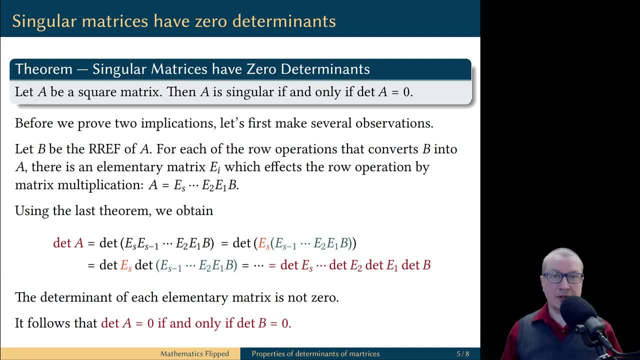 equation, all determinants of elementary matrices are not equal to zero. So this is our key observation. Let's keep this in mind: The determinant of a square matrix A is equal to zero if, and only if, the determinant of its reduced row, echelon form B is equal to zero. We are not saying: 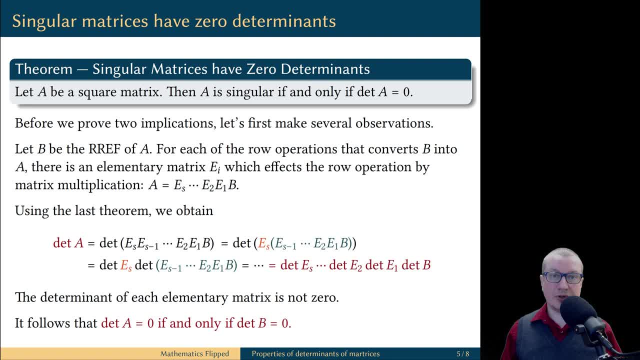 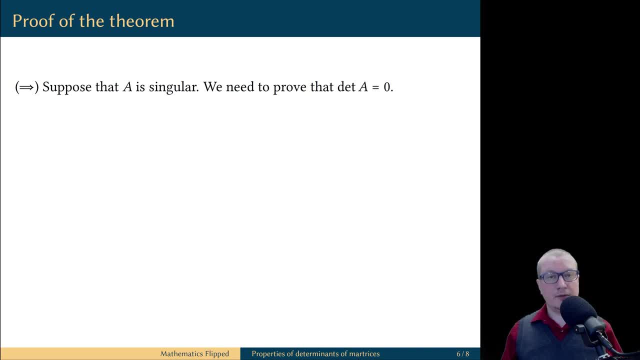 they have the same determinant. This is simply not true. But we are saying that there is zero at the same time. Now we are ready to prove the two implications in the theory. First, we are going to assume that the matrix A is singular and we would like to prove that its determinant must be. 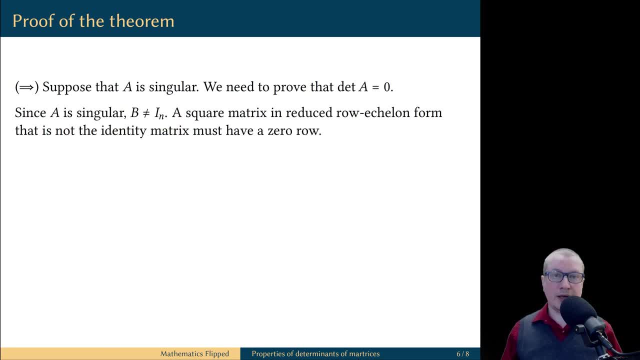 equal to zero. If the matrix A is singular, then its reduced row echelon form is not the identity matrix. But B is a square matrix which is in reduced row echelon form, yet it is not the identity matrix. It means that matrix B must contain at least one zero row. But in one of the previous videos. 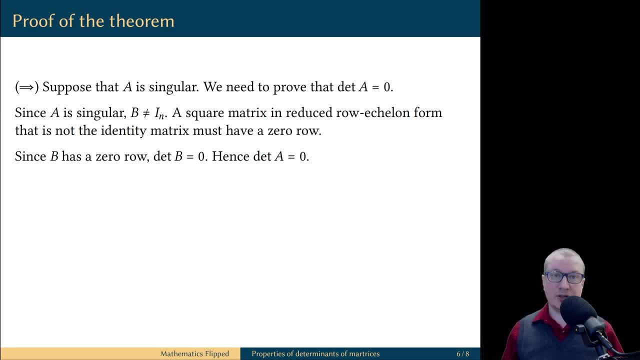 we already proved that a matrix with a zero row must have zero determinant. So determinant of B is equal to zero. This means determinant of A must also be equal to zero. In the opposite direction, let's assume determinant of A is equal to zero. We need to prove that then A. 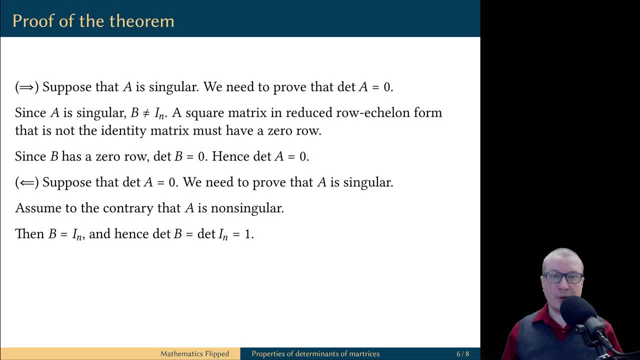 must be equal to zero. This is going to be proved by contradiction. Let's assume that A is actually non-singular. Then its reduced row, echelon form, B, is the identity matrix And the determinant of the identity matrix is equal to one. In other words, it is not equal to zero. But if determinant of B is not equal to, 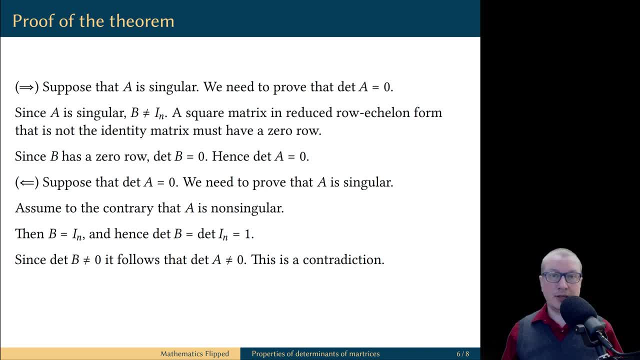 zero, then determinant of A cannot be equal to zero. This is a contradiction to our assumption that determinant of A is zero. This is a contradiction to our assumption that determinant of A is zero. This contradiction was caused by us assuming that A is non-singular. Therefore, this is impossible. 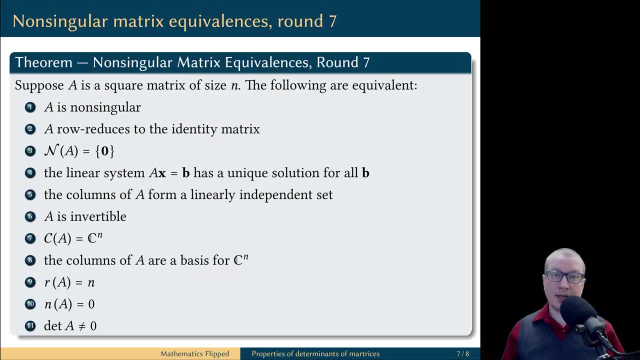 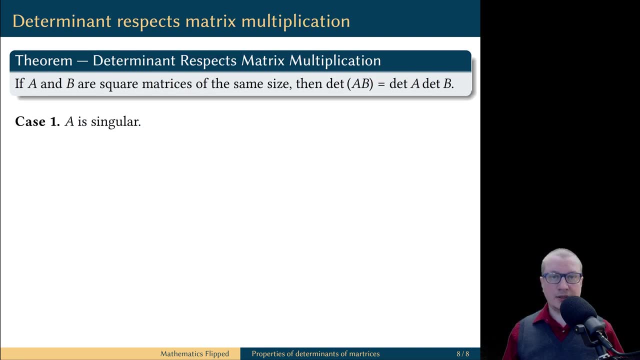 and hence A must be a singular matrix, Because this was an if-and-only-if condition. we can also say that a square matrix is non-singular if, and only if, its determinant is not equal to zero. Our last result is a remarkable observation: that determinant of B is not equal to zero. 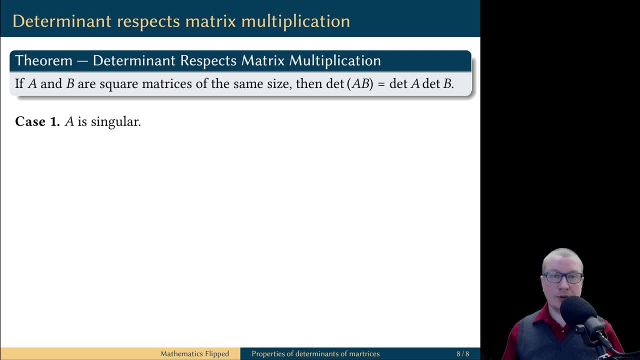 The determinant of the product of two matrices, A and B, is the product of their determinants. Notice in this equation: on the left-hand side, it's the operation of matrix product. On the right-hand side, it's the operation of the product of numbers. 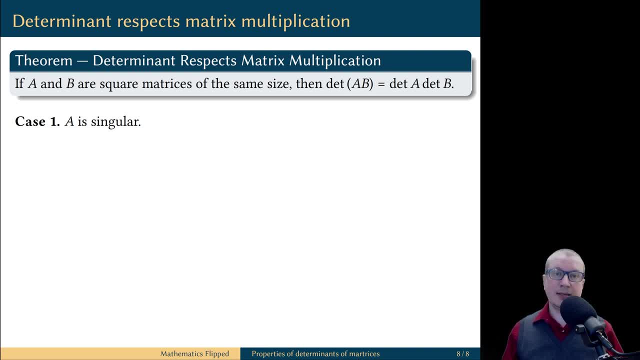 This proof is going to be proved by cases. In the first case, we are going to assume that matrix A is singular. Then its determinant of B is the product of their determinants. The determinant must be equal to zero. Also, in one of the previous videos we have proved: 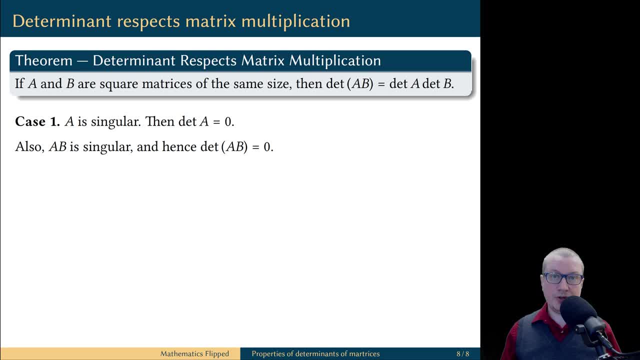 that a product of matrices is a non-singular matrix if, and only if, all individual matrices are non-singular. This means the product A times B is a singular matrix because at least one of the terms A is a singular matrix. But, being a singular matrix, the matrix AB. 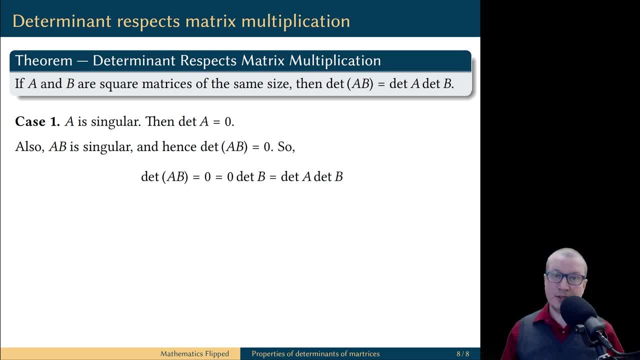 must have zero determinant. And now we see that the formula holds in this case, because determinant of AB is equal to zero, which can be expressed as zero times determinant of B, regardless of what determinant of B is, and we also know that zero is equal to determinant of A. 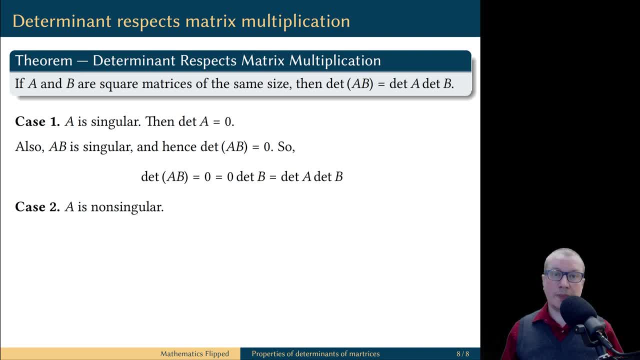 The second complementary case is when the matrix A is non-singular, Then A can be expressed as a product of A. The second complementary case is when the matrix A is non-singular, Then A can be expressed as a product of A. So to compute determinant of the matrix product AB. we are going to replace the matrix A. 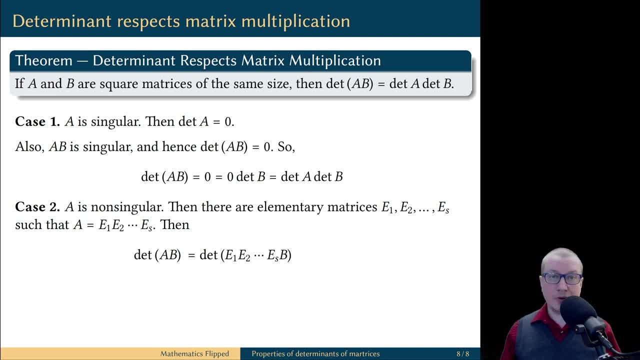 by the corresponding product of elementary matrices. We are going to chip out one elementary matrix at a time from the left and we will arrive to this product of determinants. Now comes a creative trick: Let's reverse this process of chipping out one elementary matrix at a time on the left.